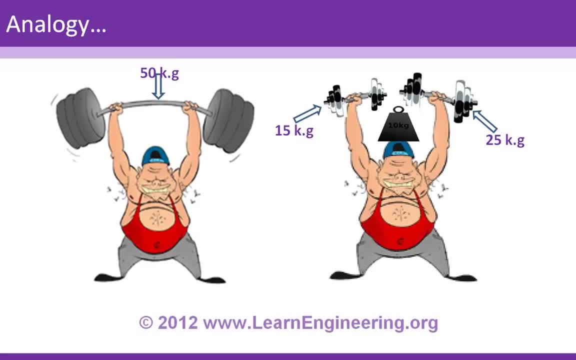 consider the same weightlifter in a different scenario. There is this: He is again lifting 50 kgs here, but in different fashion: 15 kgs on one hand, 25 kgs on another hand and 10 kgs on his head. 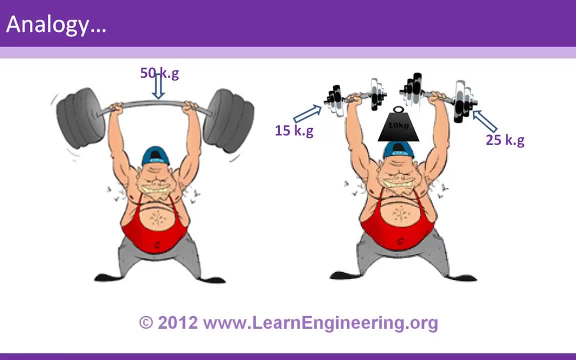 So in first scenario, we know 50 kg is the maximum lifting ability of this lifter. So is it true to say, in second case also, he won't be able to lift more than 50 kgs? It's not exactly true, right, but it is pretty. okay, A pretty. 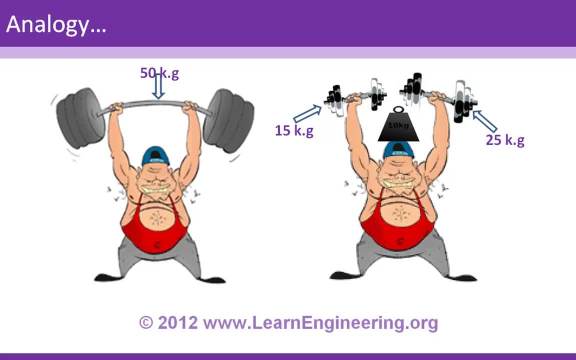 good assumption. So, if you can assume so, this will be known as a theory of failure for a weightlifter. So what we have done just now, We had a simple loading for a weightlifter and we found a maximum limit for the weightlifter and 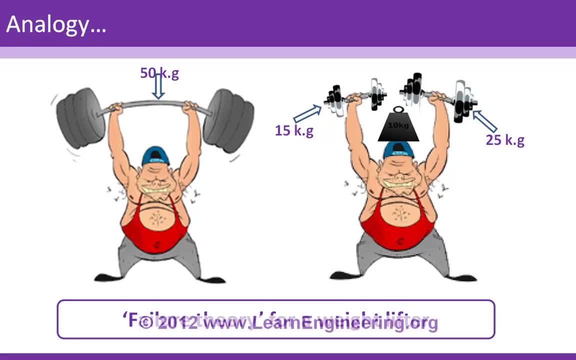 in second case you had a complicated or complex loading for the same weightlifter And we assume that the first simple loading case is applicable for the second complex loading case also. So this is all about theories of failure In material failure also. we will proceed in the same fashion, So we'll go. 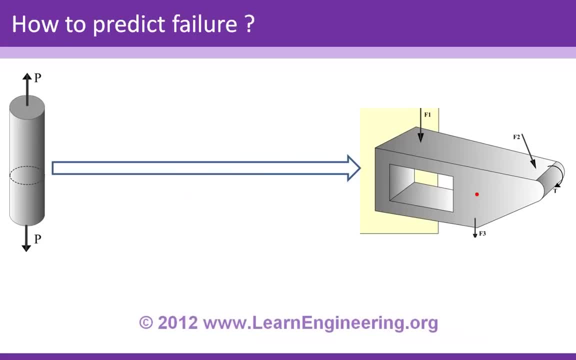 across it. Here it is. So I have got two cases here. First is a simple loading case, Second is a complex loading case. So you can well understand. first case is a simple tension test case that you perform in laboratory and results are well available and just like the weight lifter, 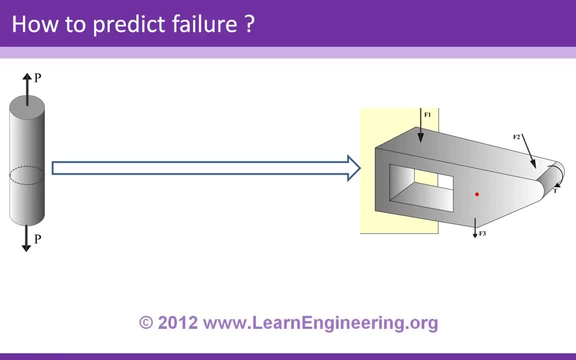 case. here also, you know at what load condition my material will fail under simple tension test and using this data you will be able to predict, under compress loading condition also, how my material will fail. so this is the way we are doing it: from simple tension test we know what's the. 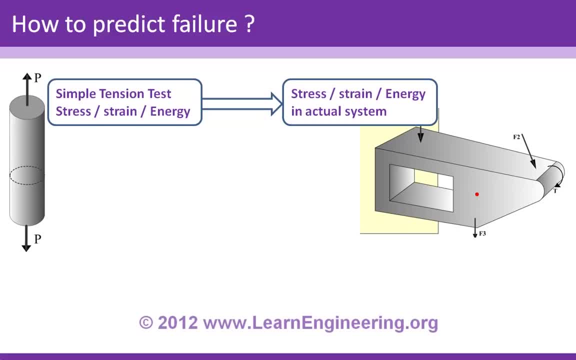 maximum stress material can withstand, or what's the maximum strain it can withstand, or what's energy stored during the failure. using this data, you will predict, under complex loading condition, when the material will fail, what you will do. you will just compare these two values. you will say: 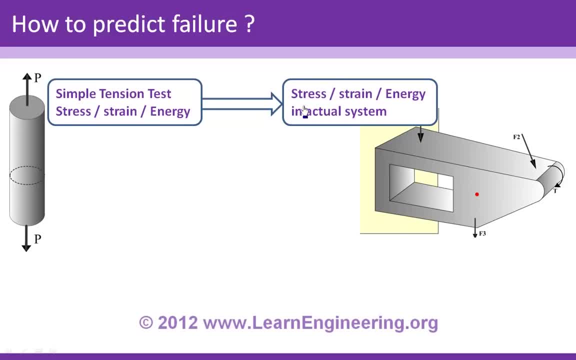 when maximum stress of my complex case exceeds the maximum stress of simple tension test, my material will fail. so similarly you will do for other variables also. so that's a concept of failure theory. but before proceeding to the failure theory is better to understand two concepts. you will need to understand the concept of failure theory and the concept of stress. of failure theory. 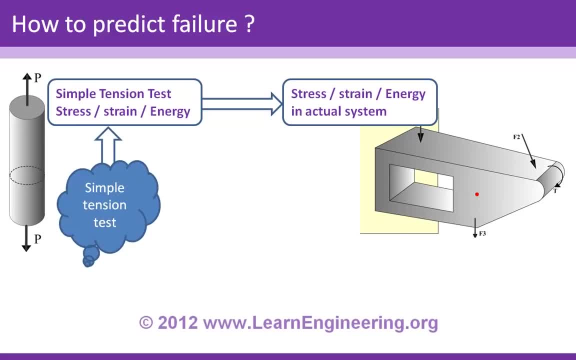 in a better way. first is about simple tension test. we will go across it in more detailed way. second, I told we'll compare maximum stress or maximum strain in a complex loading case. so in order to find this maximum stress or maximum strain in a complex situation, you have to. 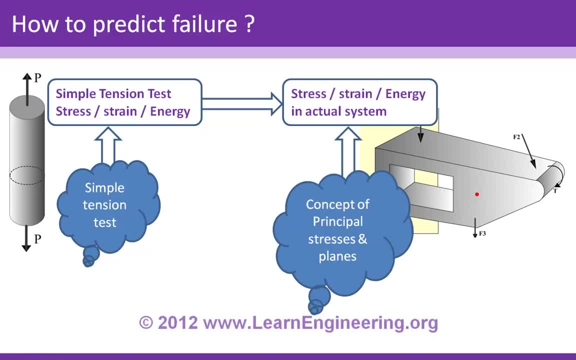 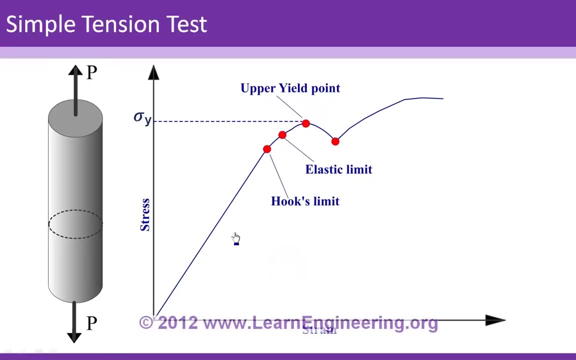 understand something called principal stress or principal plane, so we will go across this also. so, after covering these two topics, we will see what our failure theory is. so first, a simple tension test. here it is, and here you are pulling the rod with a tensile force, and it will keep on extending, and for different characteristics, as it goes on extending up to 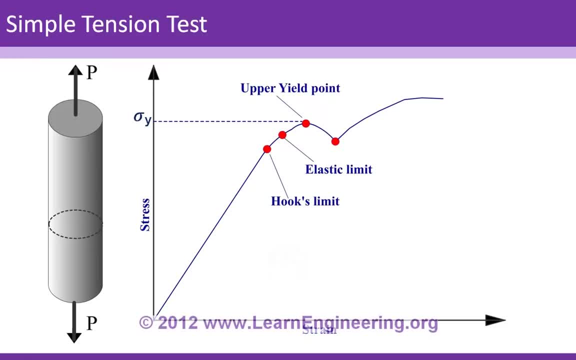 hooks limit strain induced will be directly proportional to the stress and up to elastic limit the stretch will be. elastic means: if you release, release the load from this point it will regain its original strength. but after elastic point, even if you release the force, it won't get. 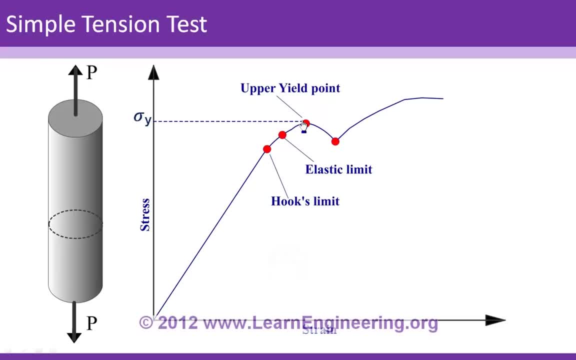 this original shape. it will undergo permanent deformation, so it's like a damage to the material. so you can well assume that elastic limit is the failure limit. after that you can assume that your material has failed. but this elastic limit is a little bit difficult to measure during a simple. 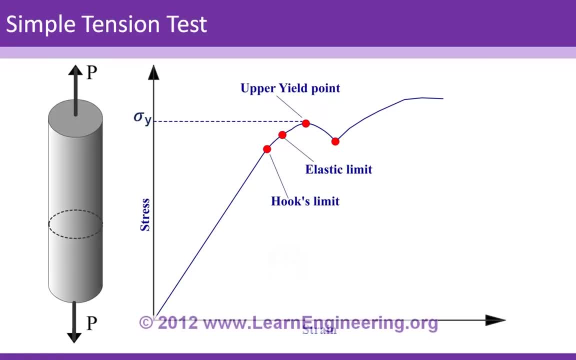 test. but just above elastic limits there is one more limit called upper yield point, where yielding- your fast deformation of material happens at this point- is easy to measure. so you will assume that the yield point is the failure criterion. or at yield stress failure of my material happens in. 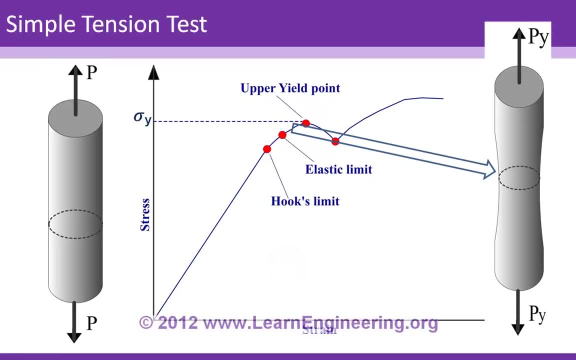 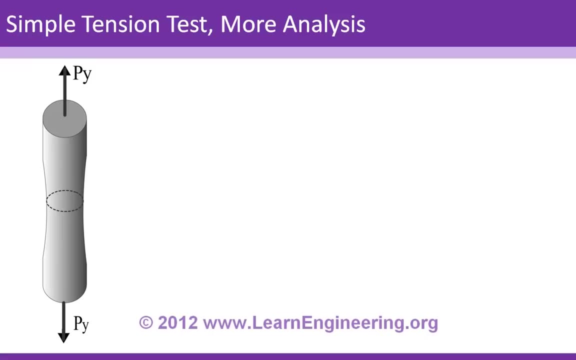 simple tension test. this is what material will look like at the time of yielding for a tactile material. it will form a neck and there will be a shape deformation to it. now we will have more analysis on simple tension test. here it is so: as your material has reached the yield limit. it 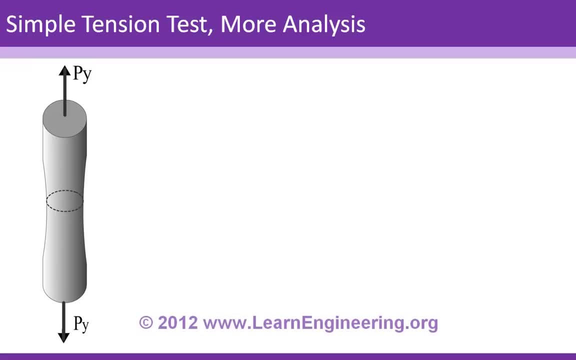 is under yielding, so force you applied is equivalent. for that now, what is the maximum normal stress induce at the time of yielding is very simple: this will be same as yield stress, because yield stress also is his normal direction. so maximum normal stress is same as yield stress. and what is the maximum normal strain at the time of yielding? maximum normal 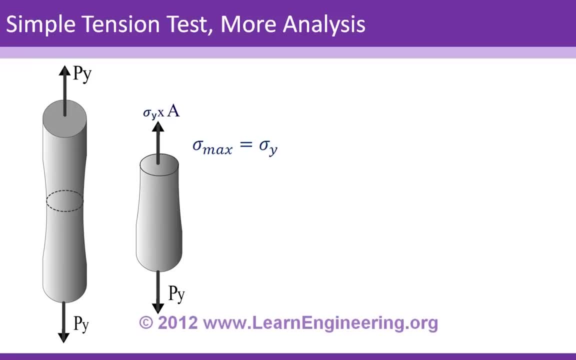 stress divided by young's modulus, you will get maximum normal strain. here it is. and what's the total strain? energy stored at the time of yielding Strain energy is area under stress strain curve, so you can well format it like this. and now, what's the maximum shear stress at the time of? 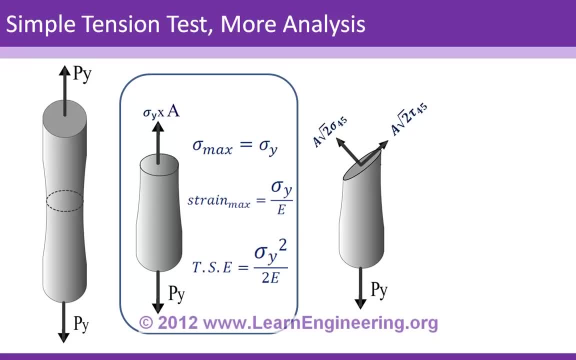 yielding and maximum shear stress happens at an angle 45 degree with horizontal like this at this location, and here is a force diagram of that and please note that area of cross section at 45 degree angle is a root 2- you can do a force simple, force balance of this diagram and you can prove that shear 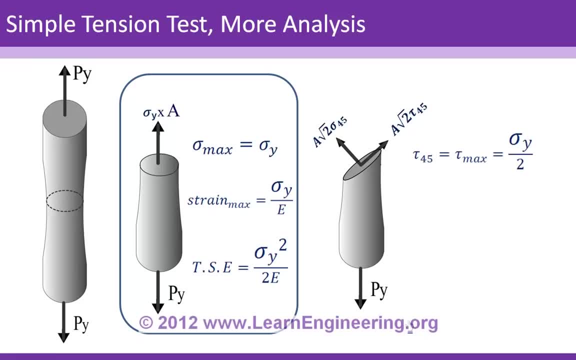 stress at 45 degree, or shear stress maxima is same as half of yield stress. the last parameter: shear strain energy stored at the time of yielding. this will be given like this equation, where G is shear modulus. now you have about five parameters in a failure theory. what I do? I will take any of this parameter and I 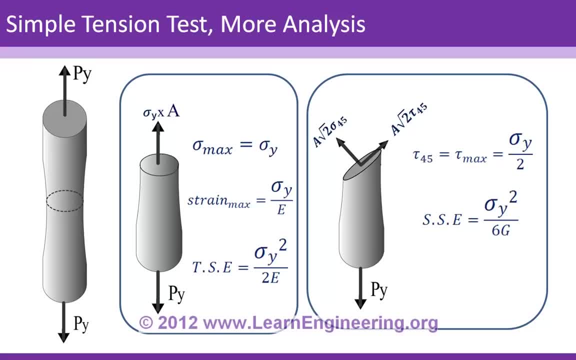 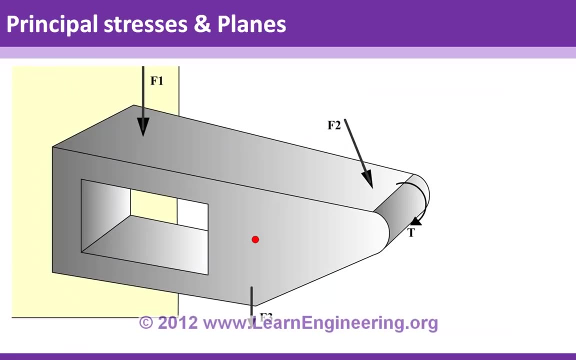 will compare with the maximum value obtained in an actual system and I will say if even my actual system, any of this value exceeds my material phase. here you have five parameters you get so you can formulate five failure theories. the next thing, to understand: the concept of principle stress. in principle plane it comes like this: this is an. 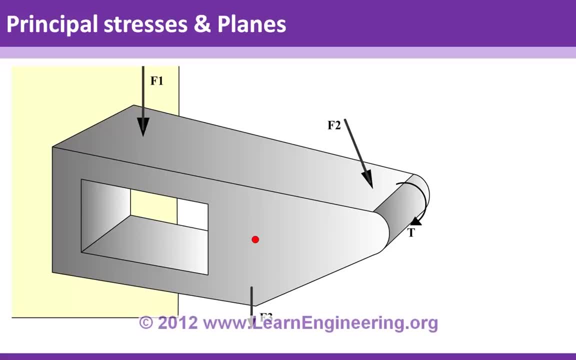 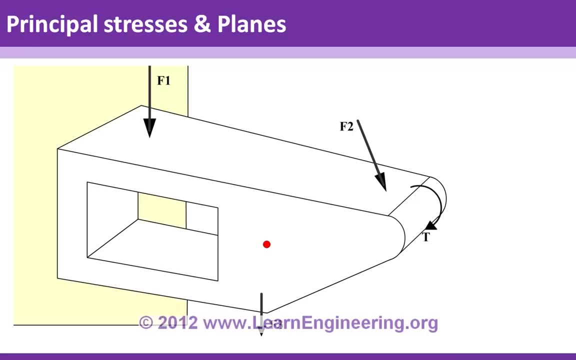 actual system under complex loading condition and I want to find out, at the red point, which is inside the material, what's a maximum normal stress induced there? or in a simple figure, it will be like this, and you know there can be infinite number of planes passing through this point, so on different planes there. 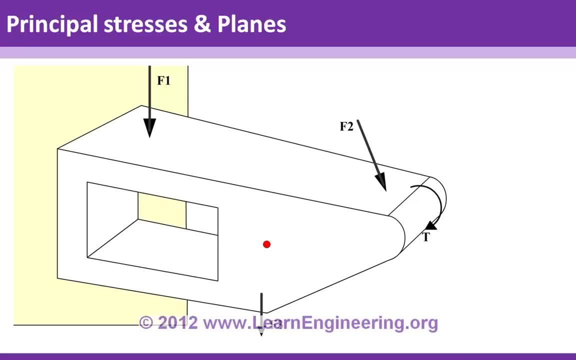 will be different normal stresses, but at one particular plane there will be maximum stress induced and this plane will be known as principle plane and stress on this plane will be known as principle stress. and if you want to find out this- values means orientation of the plane and value of stress- you have to do more circle. 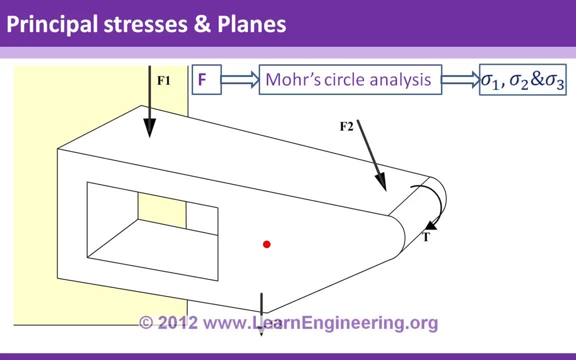 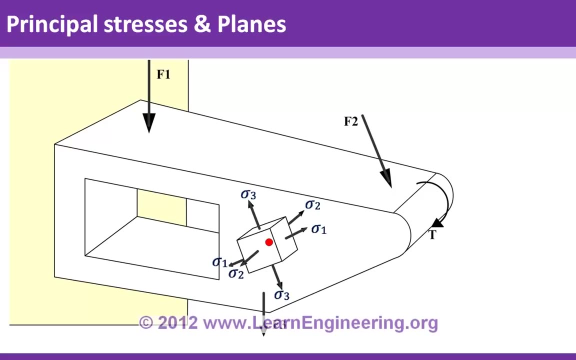 analysis where you will give force as your input and you will get principle stresses and principle plane as output. and for a three-dimensional system, there will be three principle stresses when you do more circle analysis and similarly there will be three planes, also like. this is plane number one, plane number two and plane number. 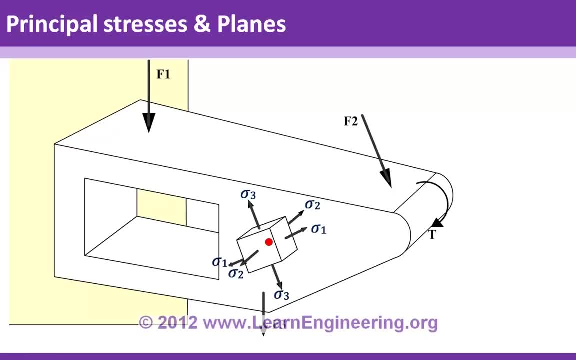 three and if you want to know maximum stress, normal stress players at this point, just compared this sigma 1, sigma 2, sigma 3 and maximum of that will be maximum normal style at that point. if funny thing and minimum of these threeständig delta, 10,000 value will be. 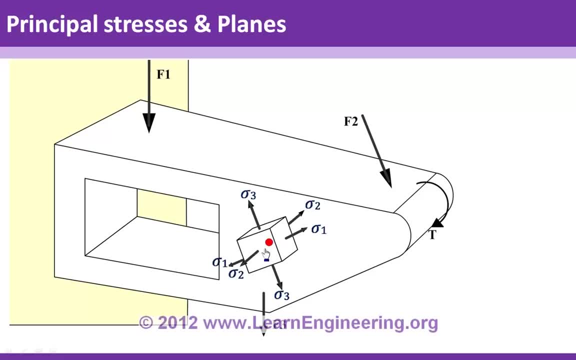 minimum normal stress at that point. and one thing to remember: on all these three principle planes, shear stress values will be zero. now we understood она once. value of maximum normal stress starts from here أ at a given point. and what about maximum shear stress value? that will be given by simple. 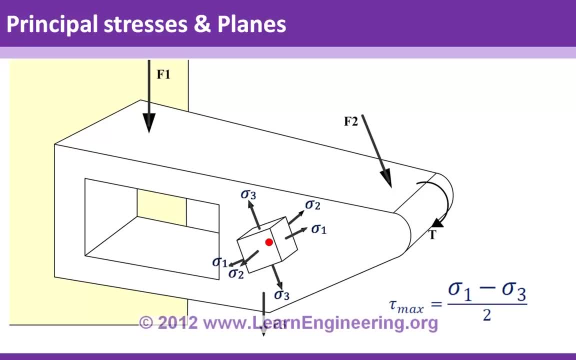 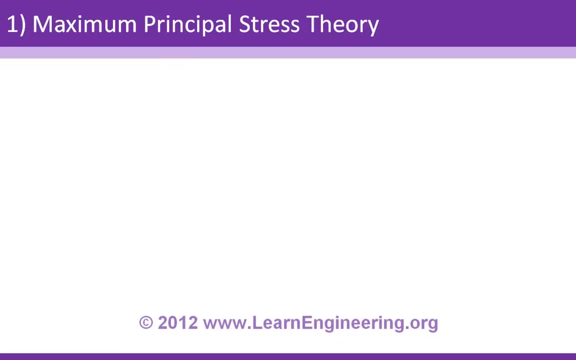 equation like this: usually we denote sigma 1 for maximum normal stress and sigma 3 for minimum normal stress. so just find out difference between these two values and divide by two. that will be maximum shear stress induced at that point. now let's go across failure theories and as i said earlier, there are five failure theories, and the funny thing is just. 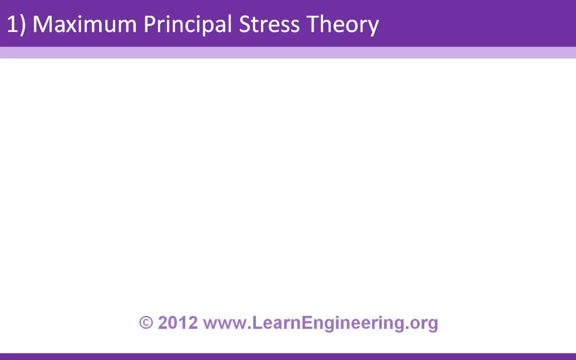 by looking at name of the theory you will be able to formulate the equation of failure or the condition of failure. here name of the failure theory is maximum principle stress theory. so, as the name suggest, my material under actual load condition will fail when maximum principle stress induced in material is same as maximum principle stress induced. 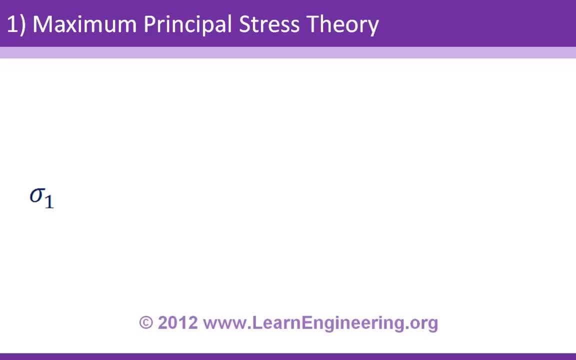 in simple tension test. so maximum principle stress in actual case is sigma 1. so if the we got from more second analysis and maximum principle stress at simple tension test is Sigma Y. so just compare this. this is a condition. under this condition, according to this theory, my material will fail, and experience has. 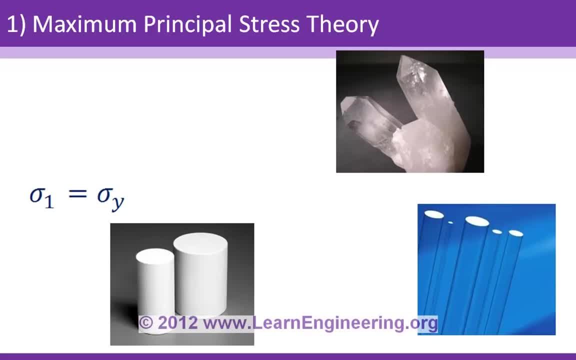 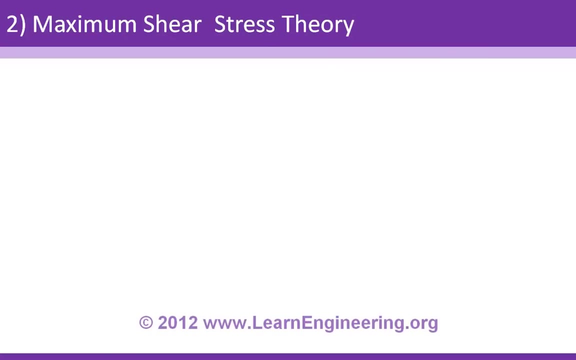 proved that this theory is good for brittle materials like glass, crystal or ceramics, but not for ductile material. if you are working with ductile material, please avoid this next theory. maximum shear stress theory has name such as it says that my material will fail when maximum shear stress induced on my 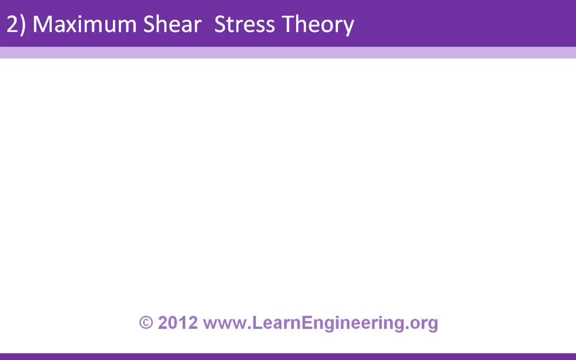 material is same as maximum shear stress induced in simple tension test and you know maximum shear stress in actual system is half of Sigma 1 minus Sigma since 3, and maximum shear stress at simple tension test is sigma 1 minus sigma 3 and maximum tension test is half a field stress. so just pick out these values and this will be the condition. 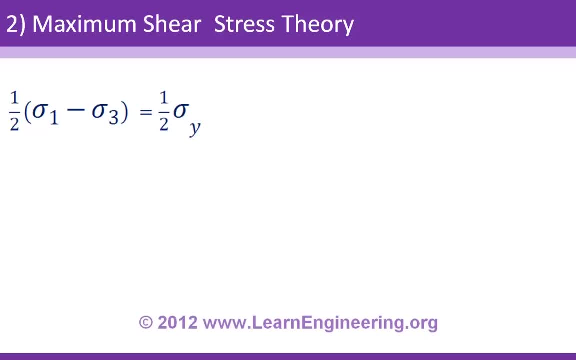 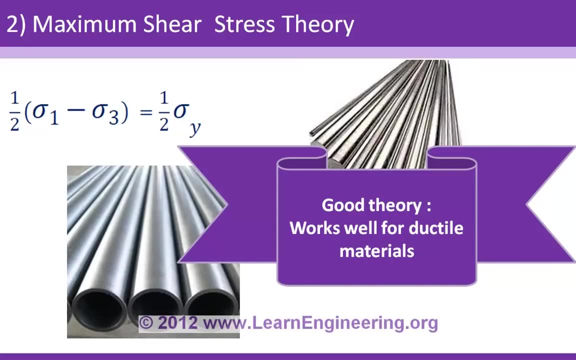 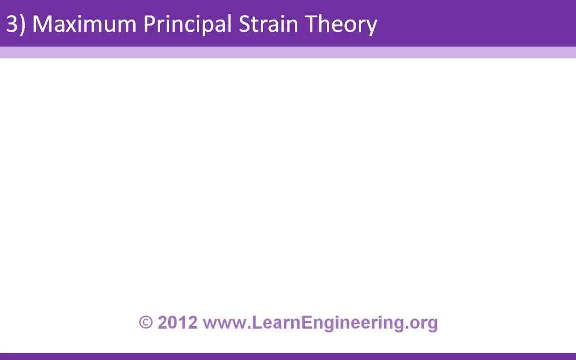 of failure. and this theory holds good for ductile materials such as steel and aluminium, and it is a pretty good theory to work with. now the third theory: maximum principle strain theory. so you can assume that when maximum principle strain in my actual system is same as maximum principle, 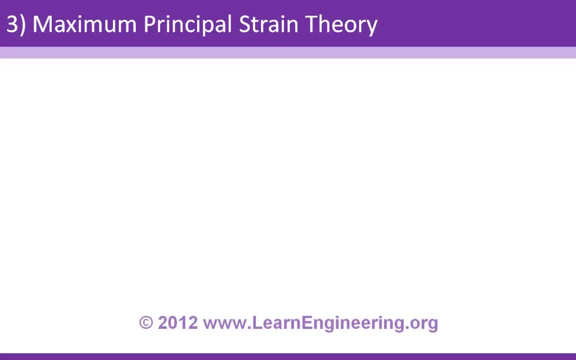 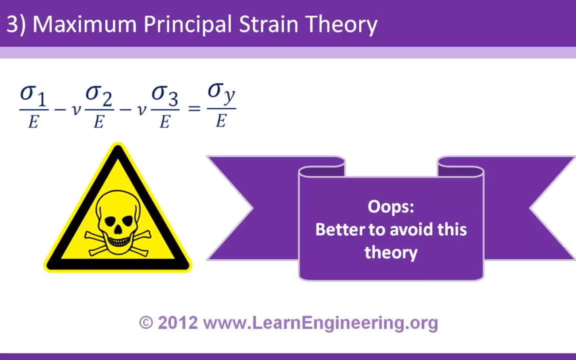 strain in simple tension test, the material will fail. maximum principle strain in actual system is like this, where mu is poisonous ratio, just to consider the effect of lateral deformation, and maximum principle strain in simple tension test is sigma y by length modulus. so this is the condition for that. this theory doesn't work for any material. 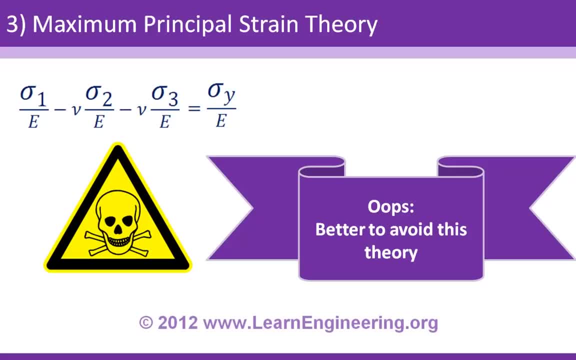 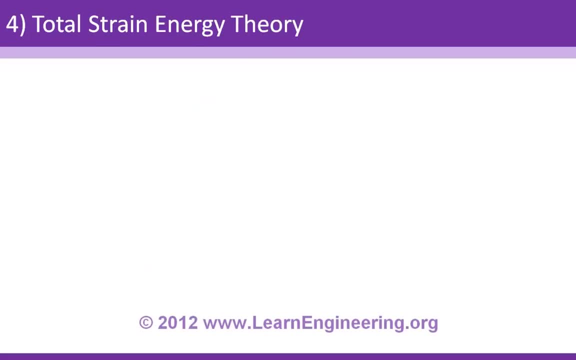 and if you use this theory for some design purpose you might end up in a wrong design, a disaster. so better to avoid this theory. now the fourth theory: total strain as a theory, here again, when total strain energy in your actual system is same as total strain energy in a simple tension, 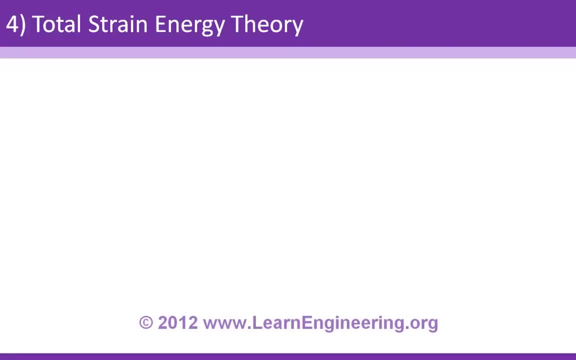 test, the material fails and total strain energy can be represented like this: a pretty complicated equation in terms of principal stresses. and you know, total strain energy in your, in simple tension test, is sigma y square by 2 e, so equate these quantities and this is a condition for failure.